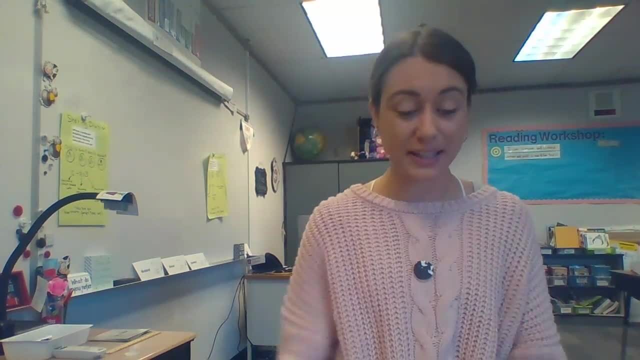 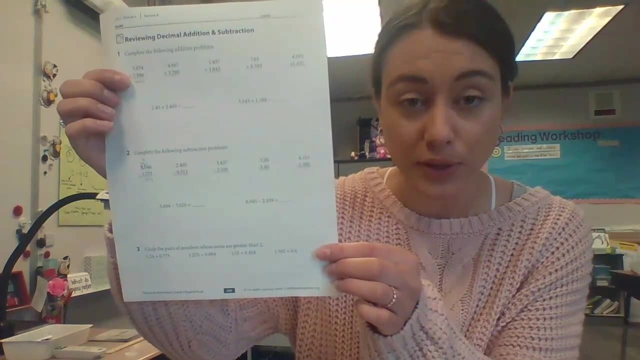 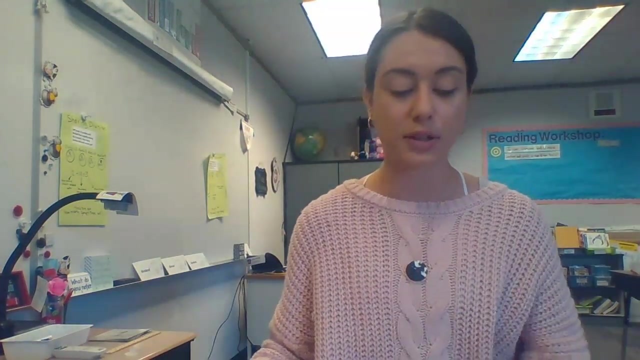 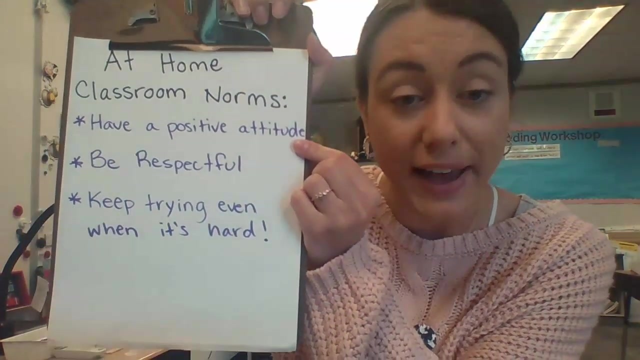 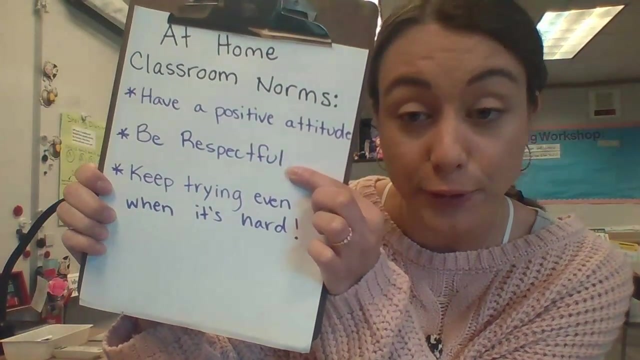 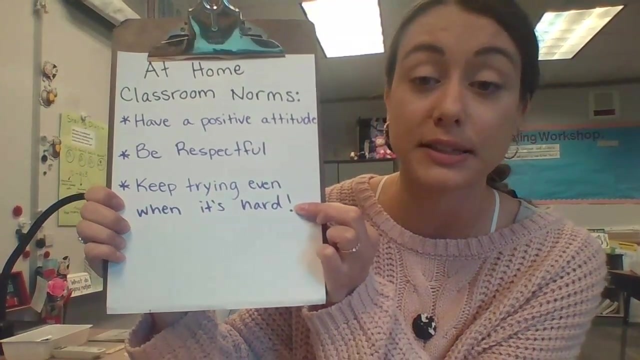 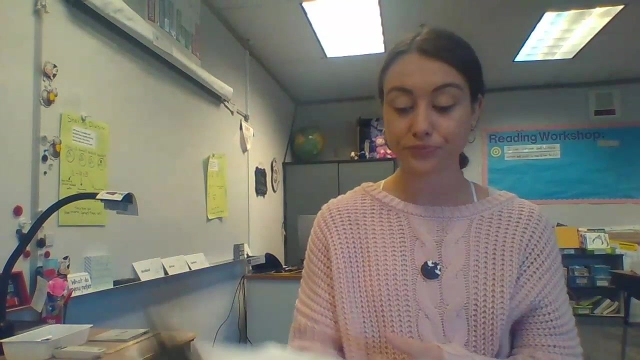 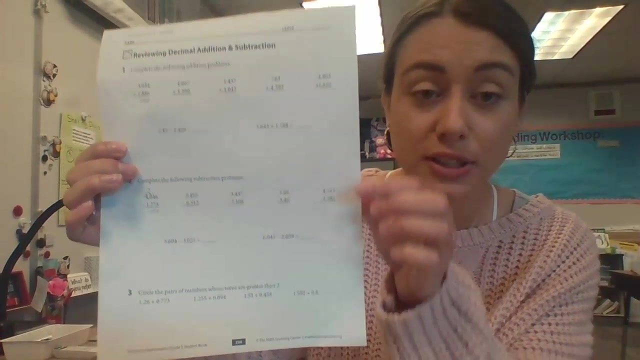 Hello fifth graders! It's Ms. Anderson here to teach you some math this week. In your packet, you have two math pages to work on. Page 298, reviewing decimal addition and subtraction, is the one that we are going to focus on in this video. Let's start with our at-home classroom norms. Our first at-home classroom norm says have a positive attitude. Make sure to be ready to learn when you watch this video. Our second one says be respectful. Be respectful to yourself and to the teacher who's teaching. Our third one says keep trying even when it gets hard. Some of these will be review, but some of these concepts will be new to you, so it's okay to ask for help when it gets hard. As you're looking at page 298, reviewing decimal addition and subtraction, you can see that the top part is all adding decimals, and the bottom is adding more decimals. As you're looking at page 298, reviewing decimal addition and subtraction, 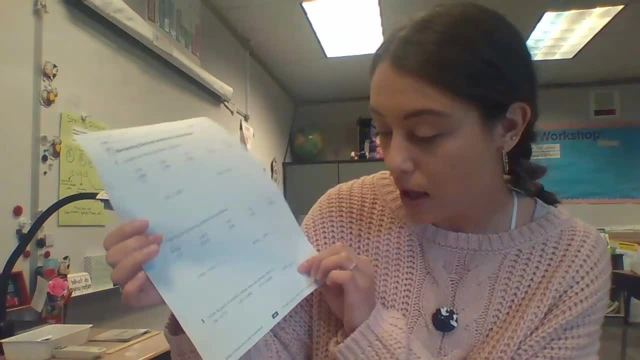 Here, number two is subtracting decimals. Then you have a mix of some more problems on the bottom. 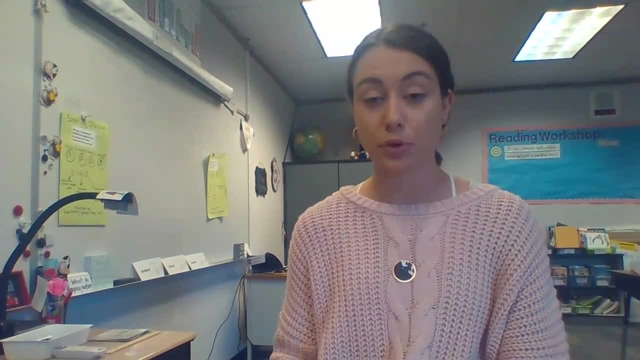 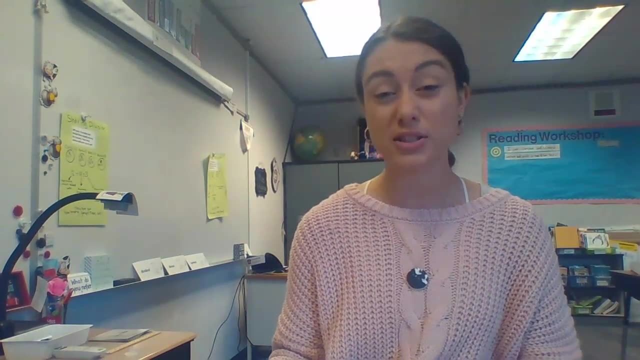 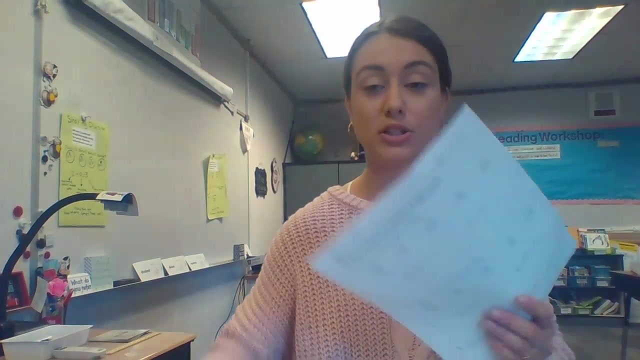 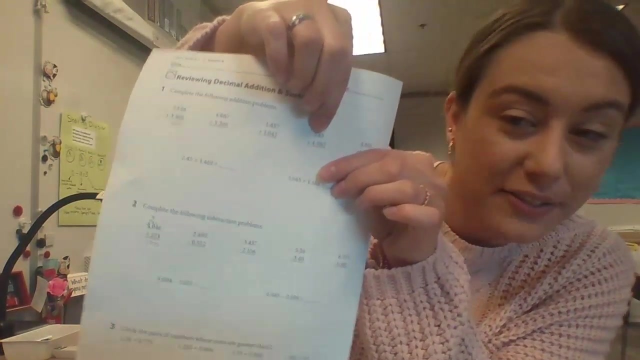 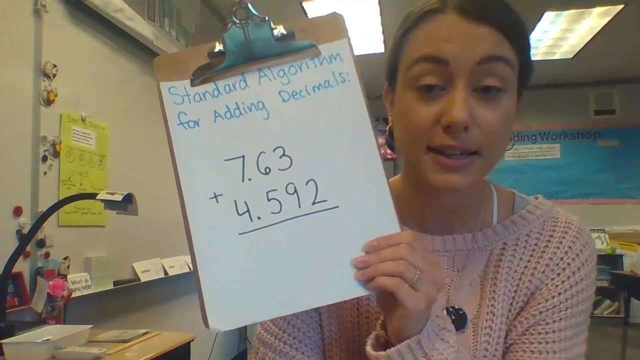 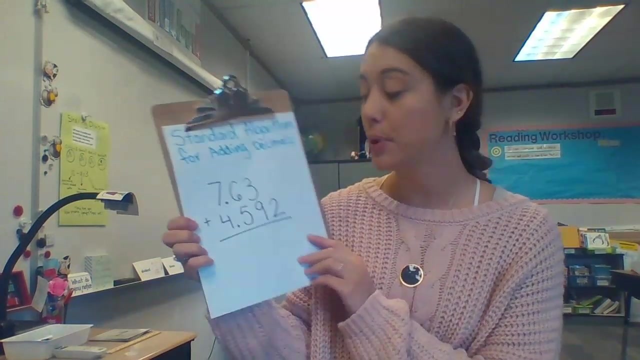 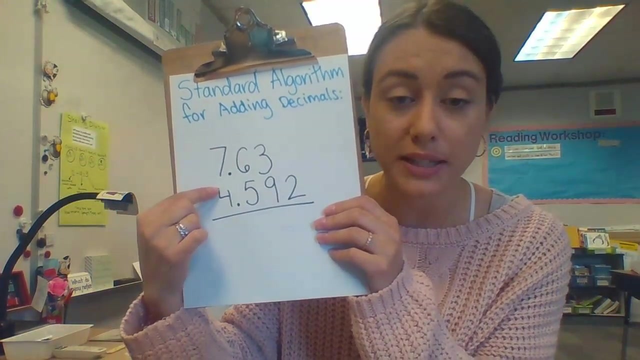 So friends, we're going to start with standard algorithm for adding decimals, and I know that the standard algorithm for adding decimals is the same as for adding whole numbers. However, I'm going to focus on one misconception that we have in fifth grade sometimes, and something that's a little bit more difficult. So I'm going to do this one all the way over here, the fourth one, or the third one that you haven't done yet. Get out your paper, I wrote it all big on a piece of paper so you can see as I am doing the work in front of you. So friends, when we are adding decimals, we have to line up the two numbers so the decimals are right below each other, or above each other. So friends, we have to make sure that the place values line up. So the ones place and the ones place, the tenths place and the tenths place, hundreds and hundreds. 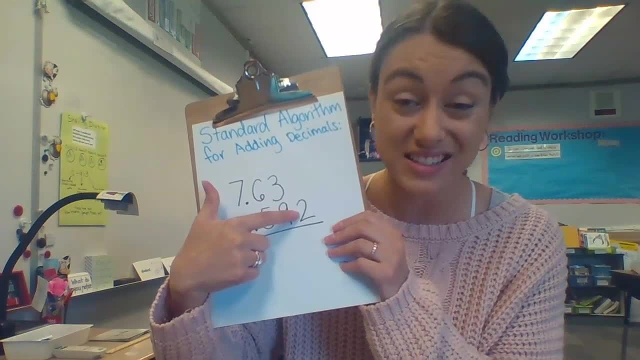 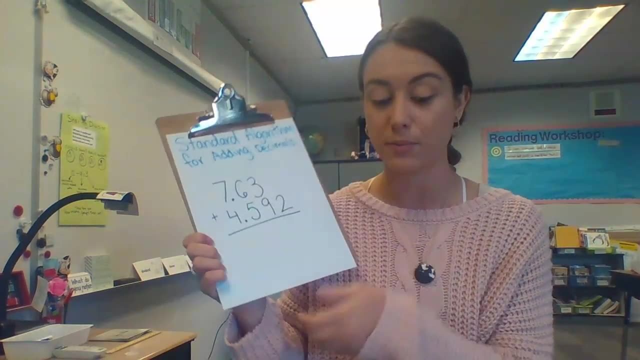 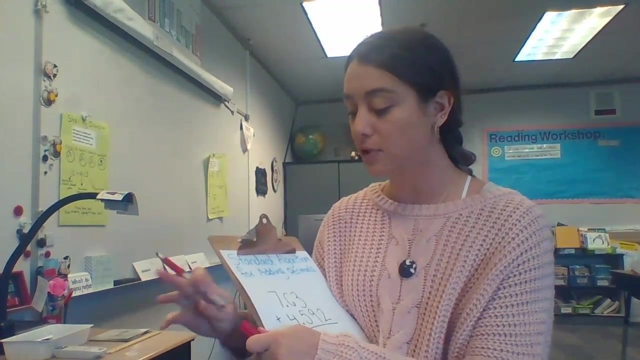 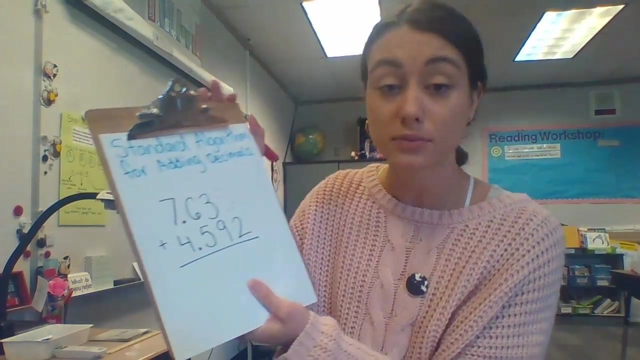 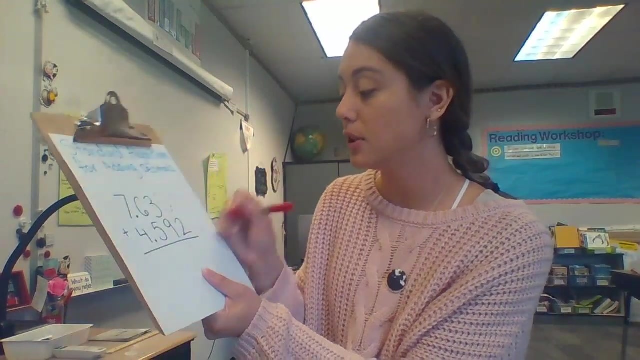 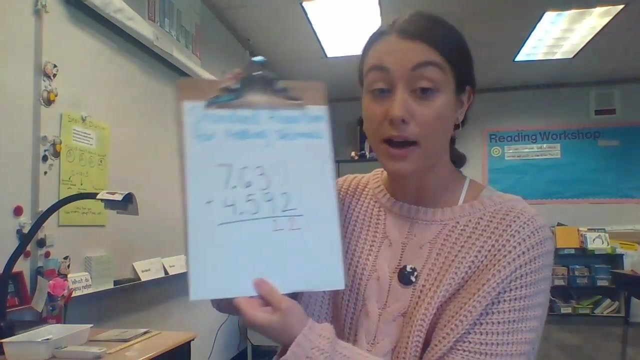 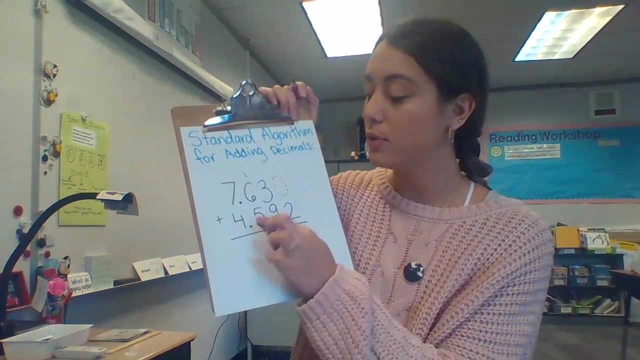 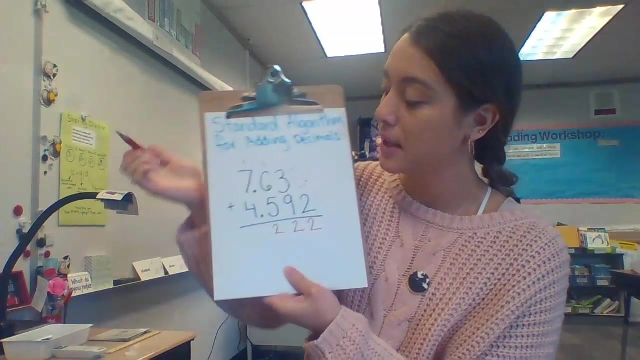 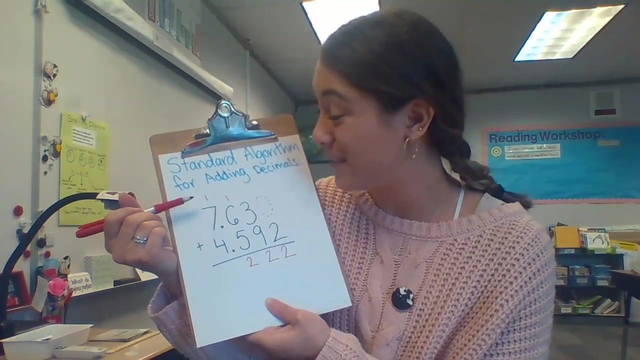 And then there's nothing in this thousands place, but there is a number in this thousands place. So we can't move this top number over, we have to make sure the place values line up when we're adding. Something that can be helpful with this is to put a imaginary zero here. You can put a zero after these numbers and it won't change the value of the number at all. So I can put like a dotted zero to be a place filler to help me when I'm adding to know what to do. So let's start with a number. Let's start adding. Zero plus two is two. Nine plus three is twelve. Five, oh, you have to carry your one. Five plus six plus one. Well I know five plus one is six, and six plus six is twelve. And then I carry my one again, and I have seven plus four plus one. Plus one is eight. Eight plus four is another twelve. 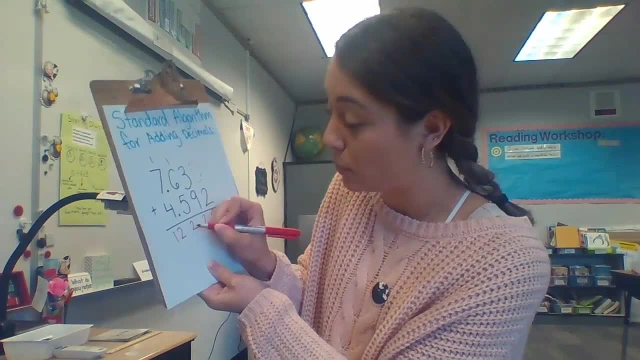 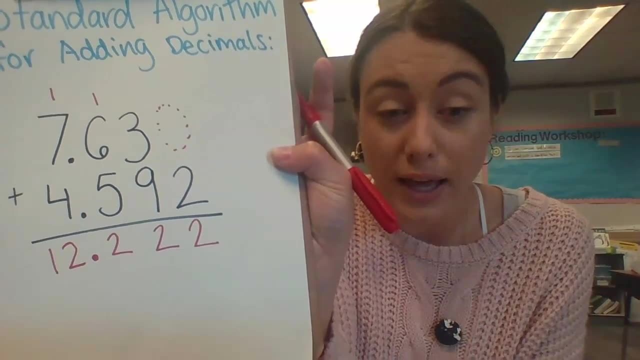 Friends, you have to make sure to bring down your decimal and put it in the same place as it was before. So you can see here my answer is twelve and two hundred and twenty-two thousandths. 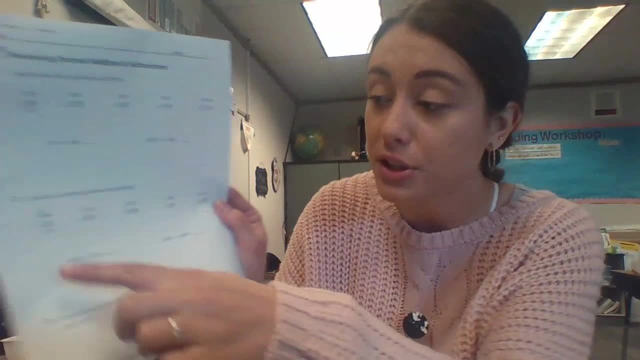 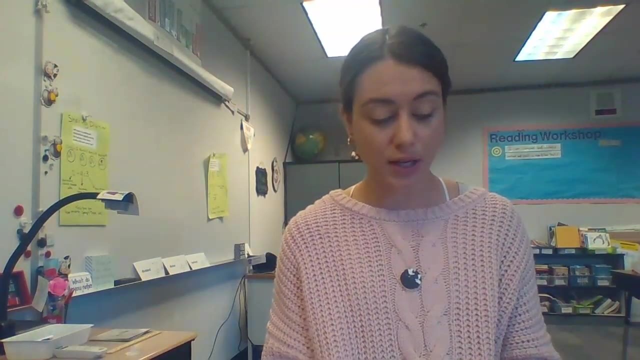 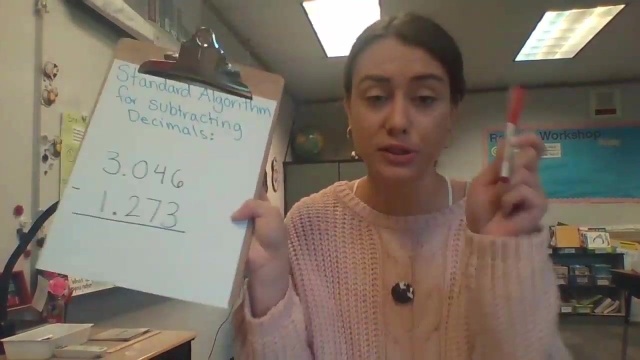 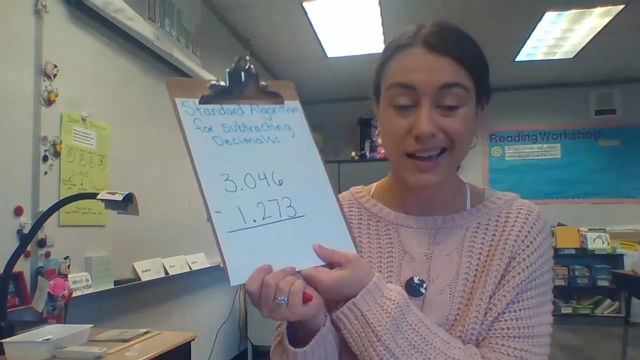 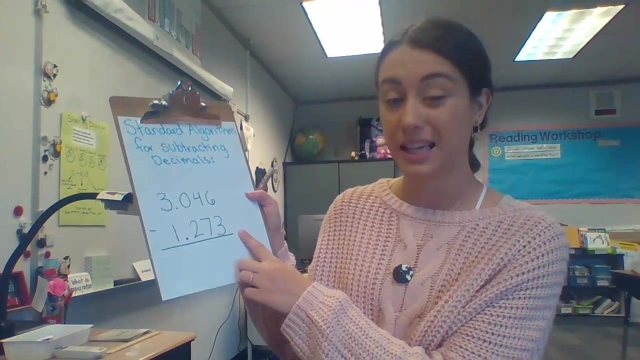 Now friends, let's work on some subtraction. I'm going to do the one that they have already given you the answer to here, and I'm going to show you how to do that one so that you know how they got that answer. I have it written blown up bigger so that you can see me do it. We're still going to use another color red to show what we're doing. So subtraction is a little bit more difficult because sometimes you have to borrow from other numbers, and that makes it a little bit confusing. So let's start just like we did before all the way to the right, and this would be the thousandths place. So we now have six minus three.